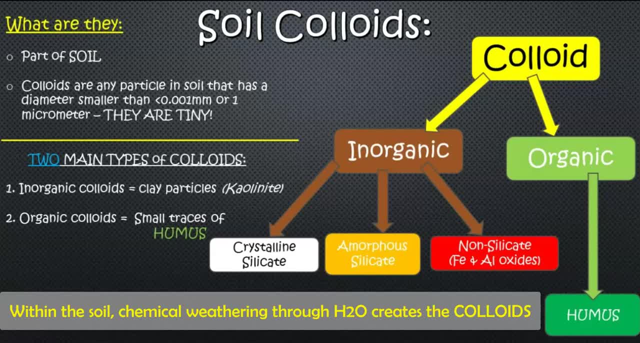 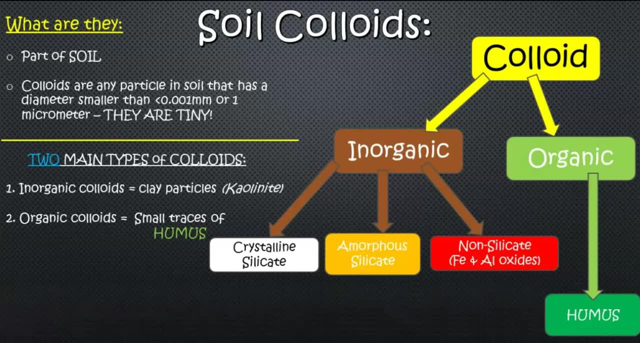 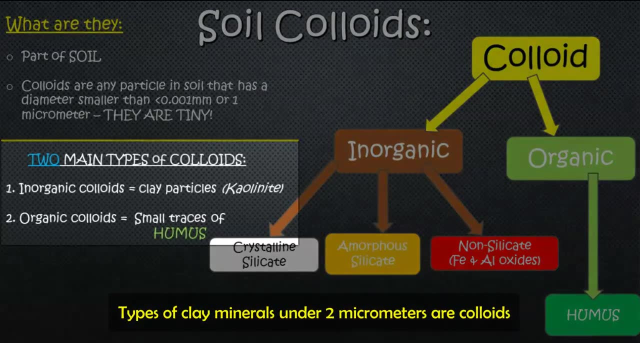 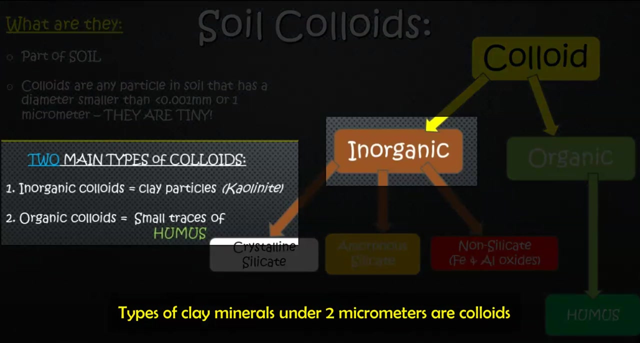 Now, in terms of types, there are two main types. You've got inorganic and you've got organic. So the inorganic, that is basically the mineral particles, and in soil the smallest mineral particle that we have or is broken down, that is in existence, is the clay mineral, Now clay particles. So the most common one is kaolinite. but there are four main types of clay minerals, based on different organizations of their silica, oxygen tetra. 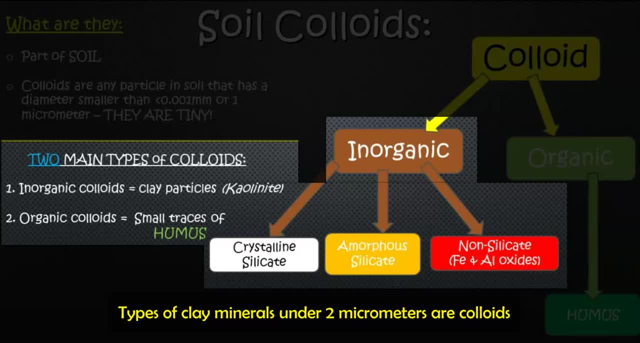 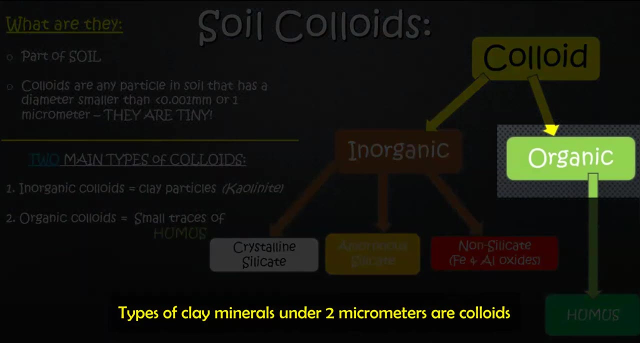 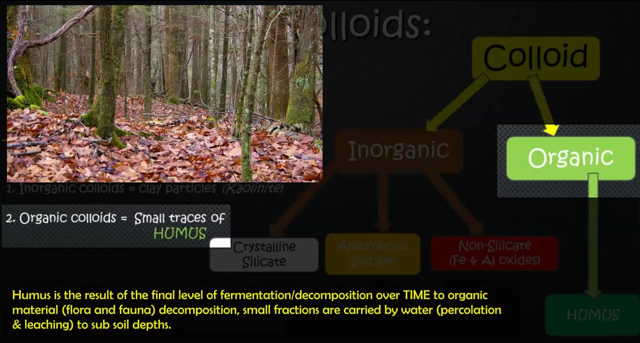 So they're polyhedral or they're polyhedral structure and they are basically the end result of all of the weathering of the materials to form these clay minerals. Then you have organic colloids. Now, organic colloids come from plant material, detritus, breaking down, decomposing material in the O and A horizon and you have the formation through different stages of decomposition, which creates humus. 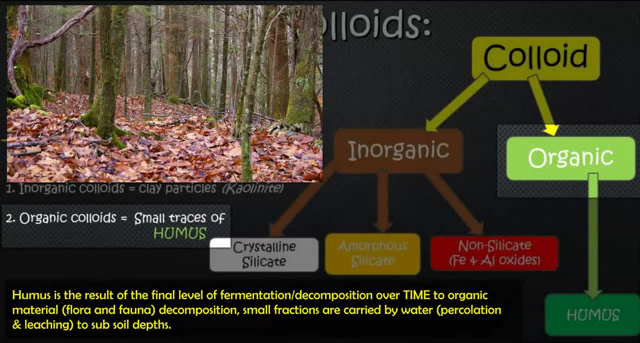 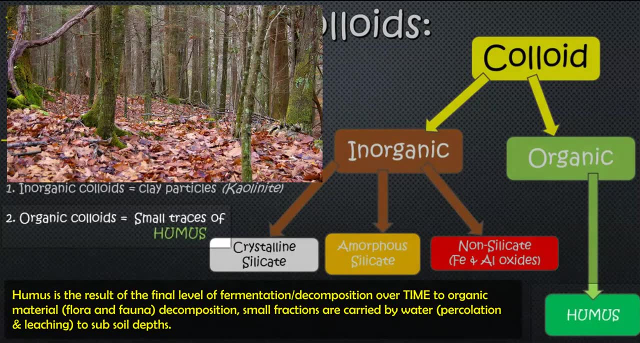 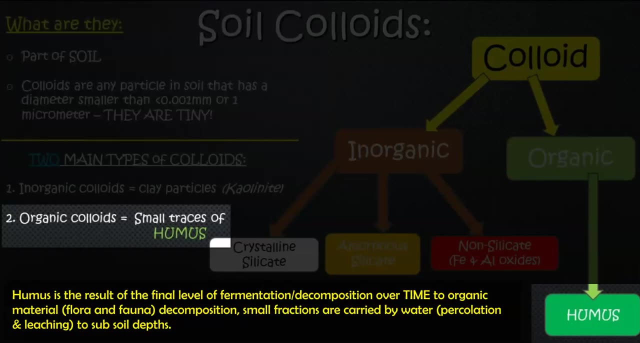 Now humus is the final stage of decomposition and you can't decompose that any further, and the small traces of this humus is the organic colloids. Now both of the colloids, both inorganic and organic, are present in solution. Now, it's not a perfect solution, so they can also be called a micelle, because they are little bits or aggregates within the solution. 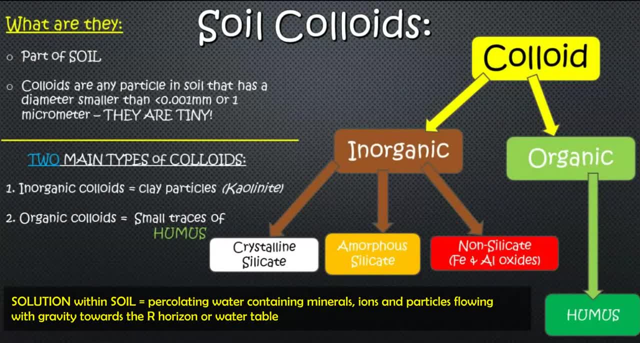 So they're transported within the solution, usually within the solution. So you have the water through leaching and percolation in the soil and it contains these little particles of either the clay minerals or the humus. So we can break down the organic into humus but the inorganic, you get these different types of clay minerals. You've got the crystalline. So when you hear crystalline you think mineral. but these are all minerals, So crystalline silicates. So you have oxygen, silicon, in the chemical formula. 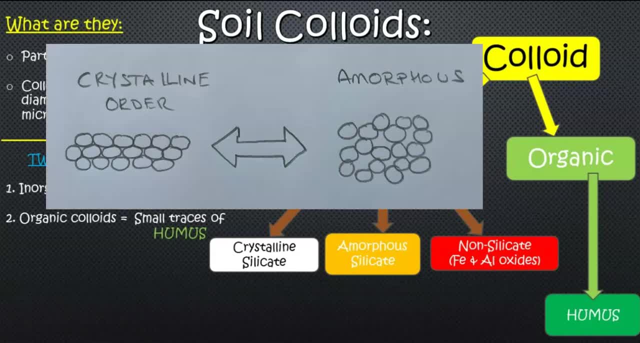 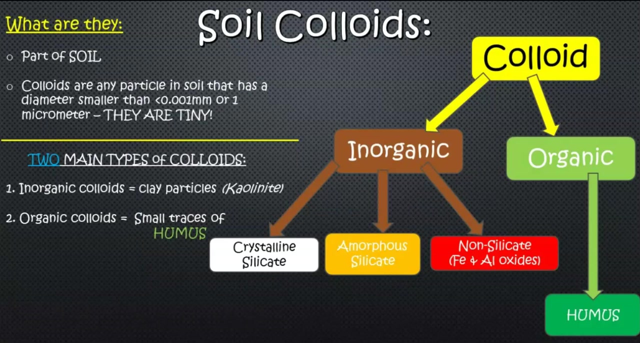 You have the amorphous. So you have the amorphous silicate, which means it's a non-crystalline shape. So the amorphous could be a different shape. Crystalline comes in a designated pattern of the elements and the bonds, whereas the amorphous could be just a generalized shape. And we also have the non-silicate, which is the iron and aluminium or aluminium oxides, which are also present in certain soils. 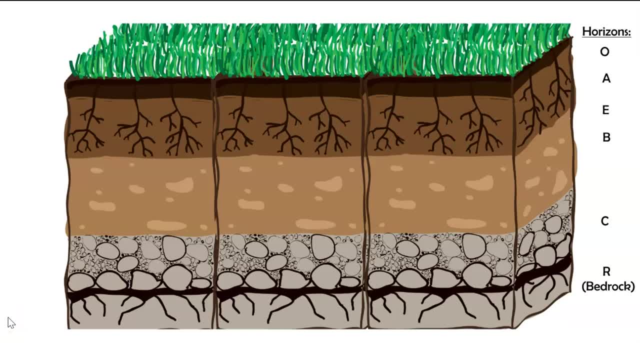 So the soil colloids, they are present in the soil as you see this soil profile here. So you have the O and A horizon at the top, with the surface horizon, with the vegetation, and you have the root system and you have this nice bedrock down here, The C horizon, B horizon, and this larger A and E horizon And the O is this very dark based on organic material. 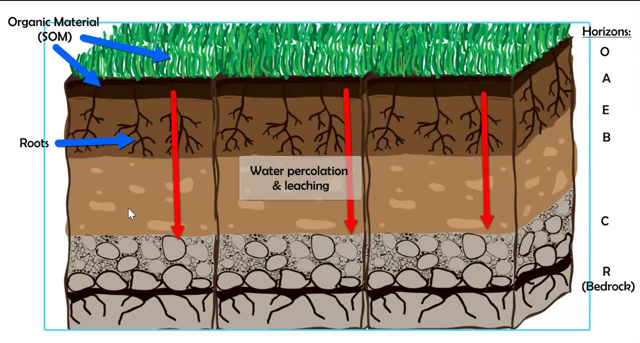 So the B horizon, that is the zone of accumulation, and E horizon is a zone of alluviation, which means that the process of leach and percolation of minerals and ions and components out of the horizon to be dumped in the b horizon right here, which is a lighter color, so it's less. 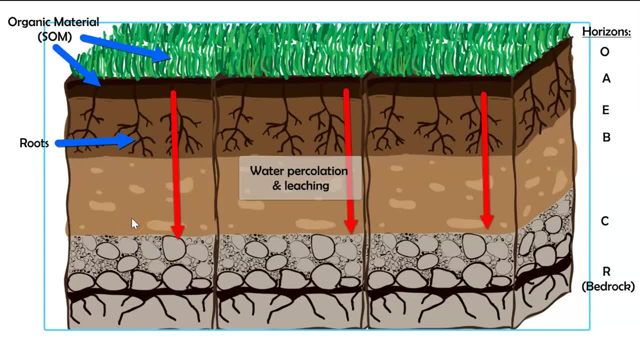 organic material as you go down in depth. so the soil colloids, they are present as a larger structure up here in the own a horizon. but when you get the physical or mechanical weathering and then you get the percolation of water, you get that in instant chemical weathering. 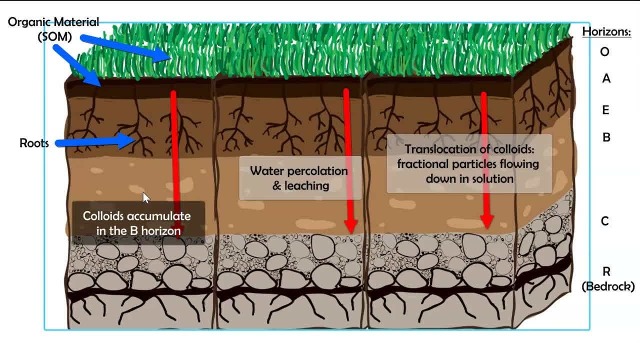 reactions with the water and hydrolysis and oxidation reduction and you get the chemical weathering going through the percolation and the water transports and translocates all these particles, both organic, which is the humus, and inorganic, which is the mineral particles, the clays. 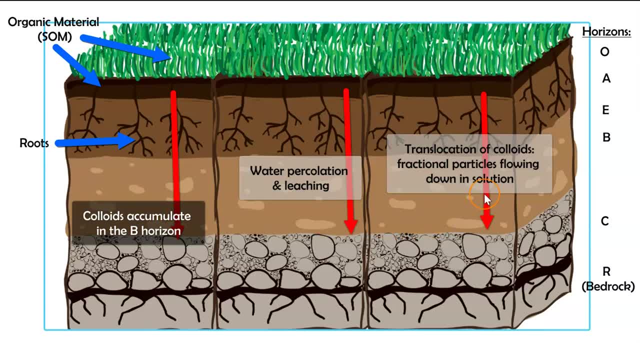 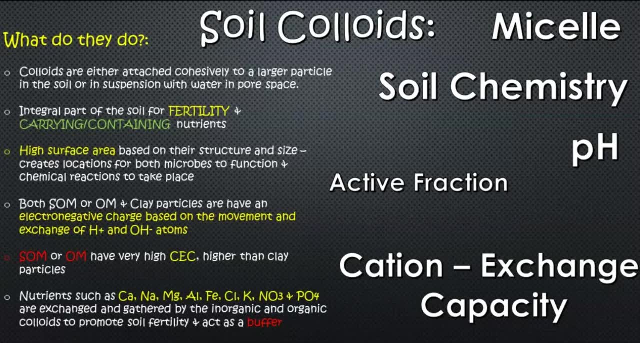 down deeper into the b horizon right here, and it accumulates and you get this large amount of soil colloids in the b horizon. so what are these soil colloids actually doing? do so once you form them, through the chemical reactions between both primary minerals and secondary minerals. a secondary mineral can be formed through chemical reactions within the soil. 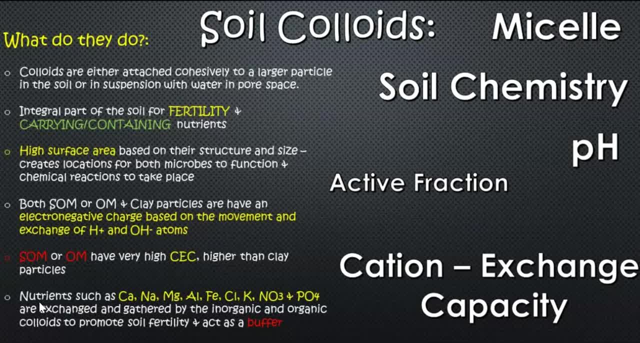 so you add in those basic elements and you start to combine them to make secondary elements and minerals within the soil. so these colloids can be these tiny particles of humus and the clay minerals. they can be attached to other like larger particles within the soil. maybe that's a larger organic material, a root nodule perhaps. 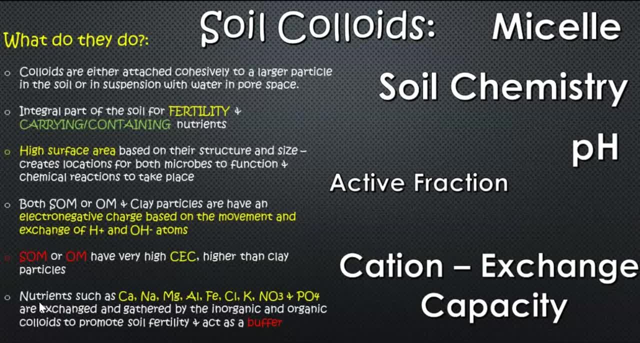 or it could also be attached to a mineral particle like a sand grain or a silt grain in the soil, or part a broken part of the bedrock in the sea horizon, perhaps as it gets broken down into the b horizon, so it can be attached and then the colloid itself has a very large surface area. so 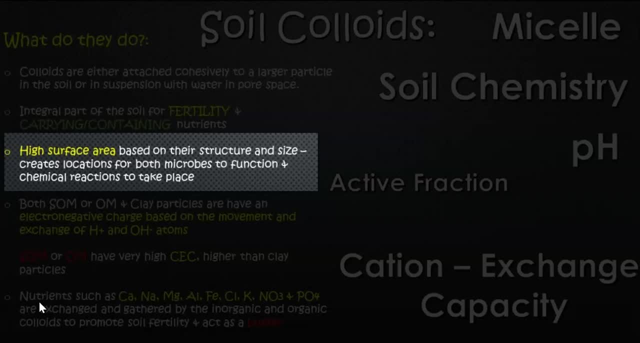 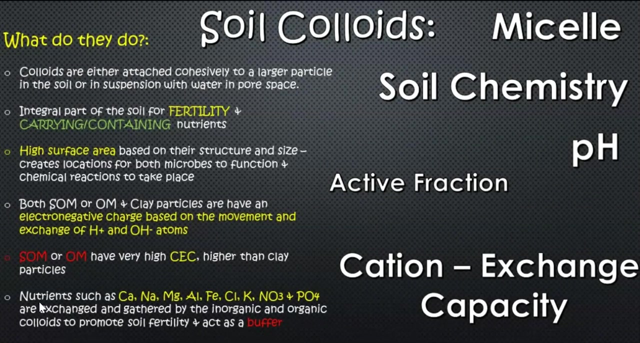 it's great for exchanging and transferring elements and ions within the soil. it's a good boundary layer of transferring elements and ions within the soil, which is perfect for soil fertility and how these colloids can contain and catch nutrients for the plant to take out of the water. so the these 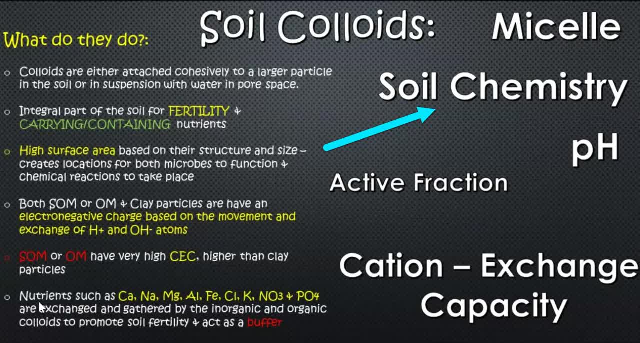 attached colloids on the particles can be exchanged and moved through ion exchange into the solution. water solution within the pores in between the particles and the organic material, like the plant roots or other vegetation, can take the colloids and take the, the nutrients and the elements out of the water that was in solution. 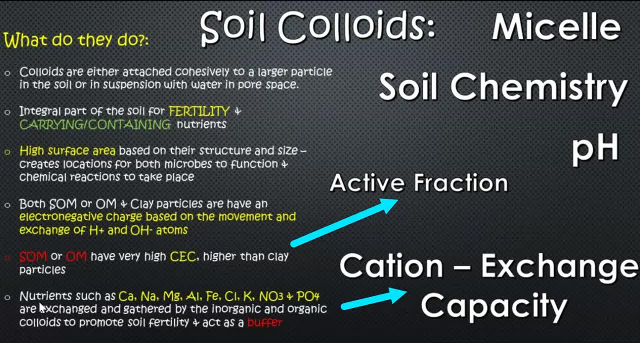 into the root system of the trees and plants and that's how the vegetation is going to acquire their nutrients and that's also the way vegetable production is going to apply for them anyway, their nutrients and also their water uptake. So this colloid is essential for 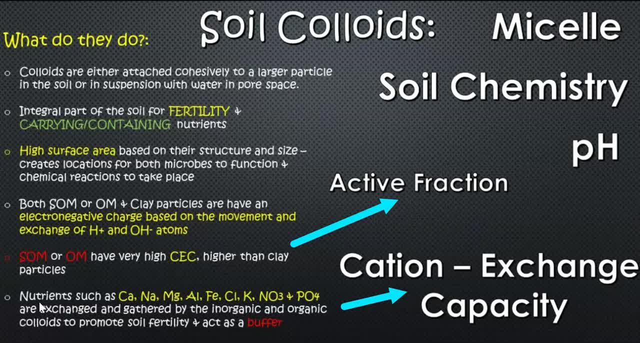 nutrient movement and basically soil fertility. So this also works as a buffer, so you can buffer the acidity of the soil based on these various elements and ions and nutrients. So pH plays a big role in soil chemistry and how the soil functions as a fertile medium for vegetation. The active fraction, that is 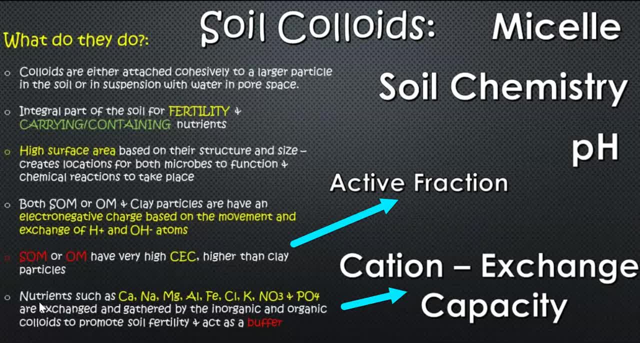 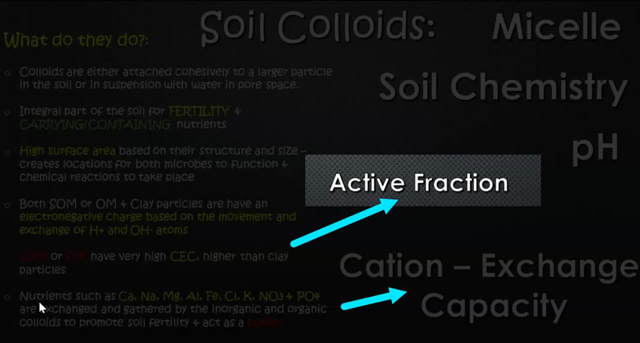 where you have a small percentage of the soil, are these colloids, a very small percentage, which is chemically active, moving ions and attracting ions and exchanging ions. So that really plays an important role in the fertility of the soil. is this movement and exchange of cations? because the colloids are?